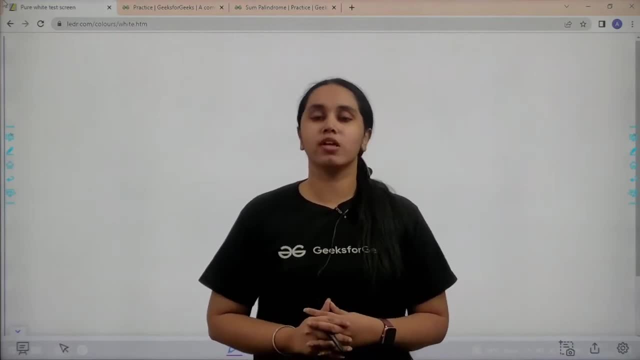 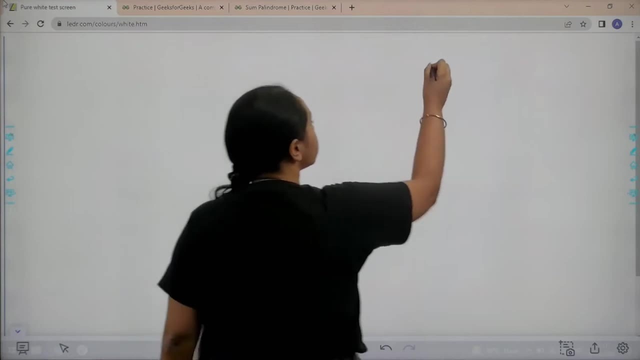 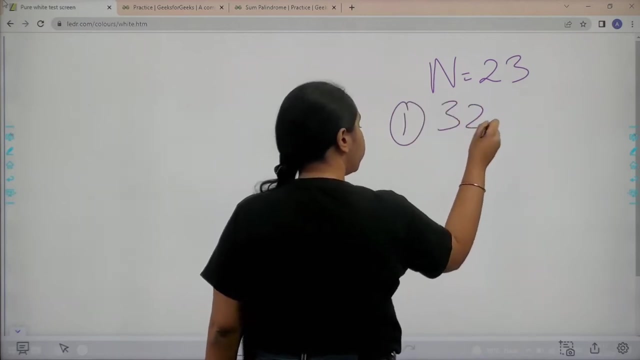 Hello everyone, welcome back. In this video you would learn how to solve the practice problem, some palindrome. So first let's understand the question. In this question you would be given a number, let's say 23.. Now first step is to reverse it. that makes it 32.. After reversing: 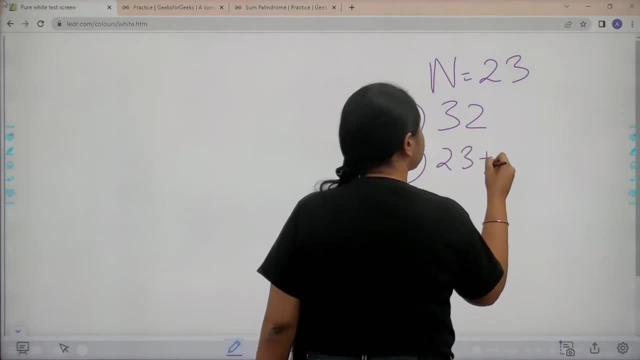 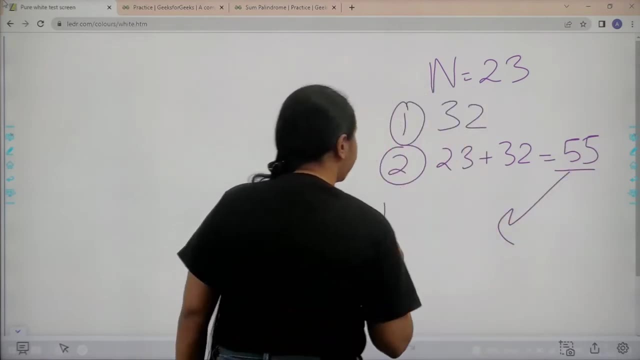 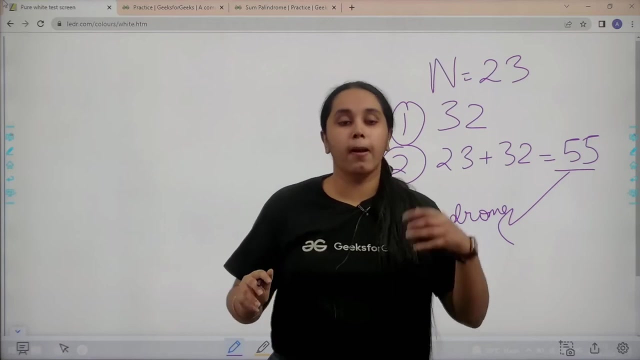 it. you need to add them together, So that is 23 plus 32. that makes it 55.. Okay, now you can clearly see it's a palindromic number, right, palindrome. So you, if, once you see if the output is palindrome, you need to stop there. But, for example, if this was not a palindrome, and let's 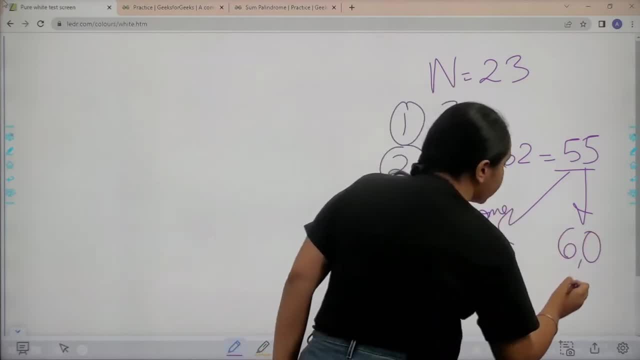 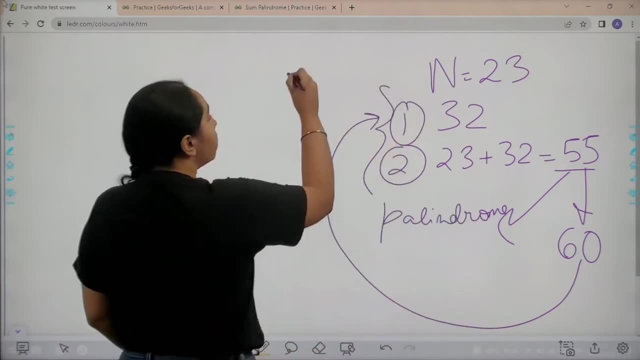 say it was 60. Okay, then what you had to do then? you need to keep on repeating these steps again and again until it becomes a palindrome or more than five iterations have happened. Okay, so there is a limit. you can only repeat these steps five times. 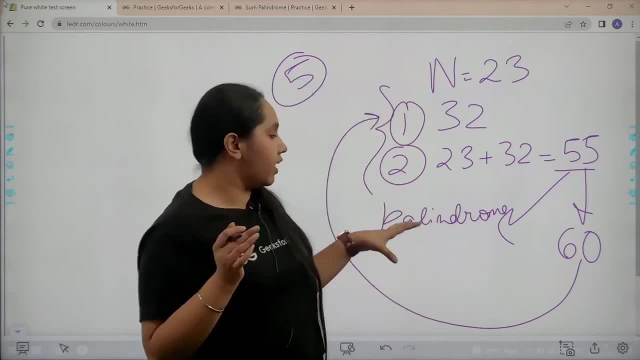 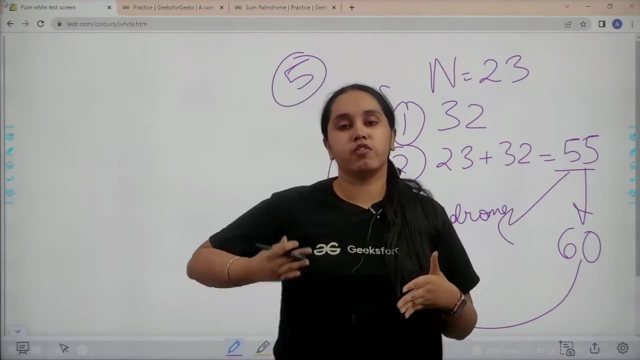 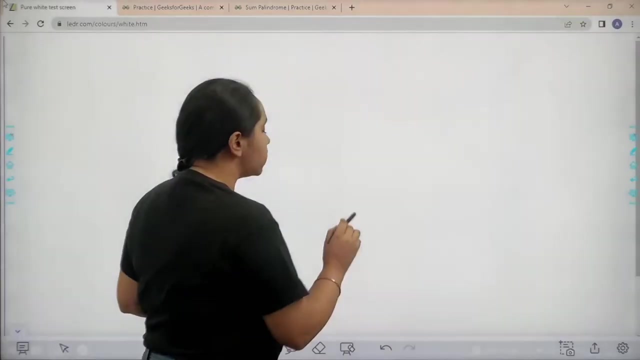 In. if those five steps, it becomes a palindrome, then it is fine, it's okay. But if it doesn't becomes a palindrome, that means you can stop there because five iterations are over. Okay, so I hope the concept is clear to you and now let's solve it. So what you need to do is you. 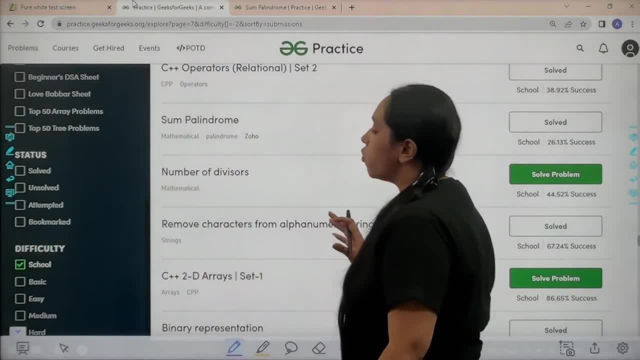 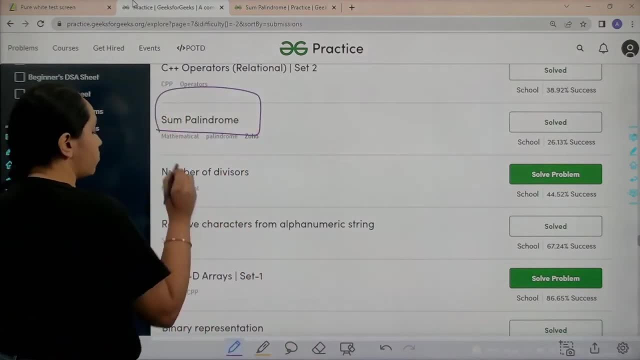 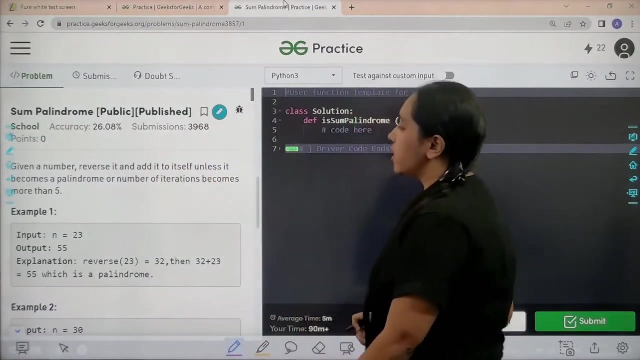 need to go to the practice portal. In practice portal, in the difficulty section, choose school- Okay. after choosing school, find the problem: some palindrome. Okay. after finding the problem, you need to click on solve. Here is the problem. let's read the statement. Given a number. 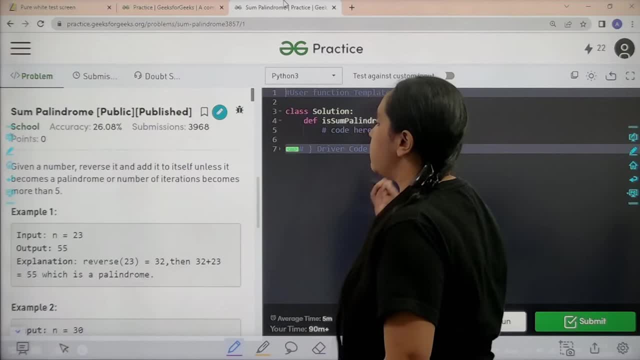 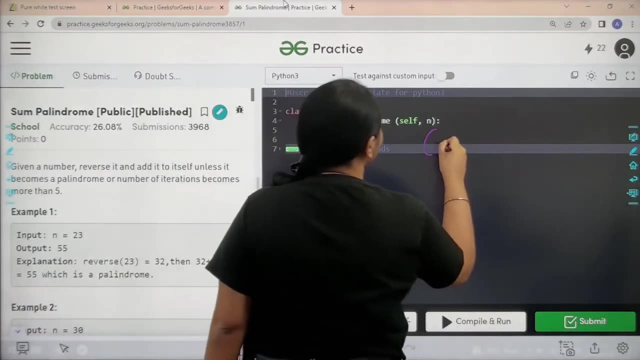 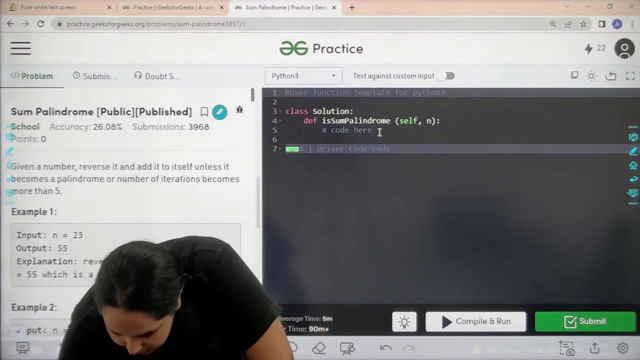 reverse it and add it to itself, unless it becomes a palindrome or number of iteration becomes more than five. Okay, now we need to code it over here. Okay, so let's start. let's solve this question. Okay, first let's say that I want num, another number, So it is. 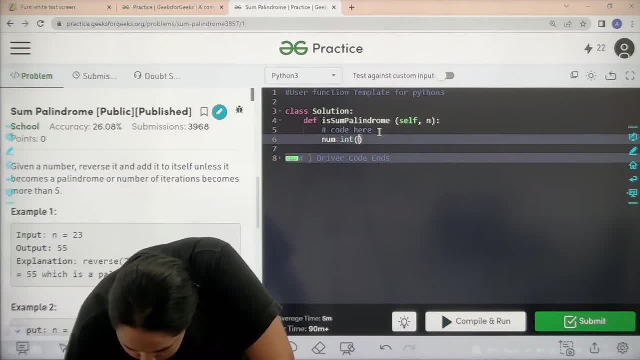 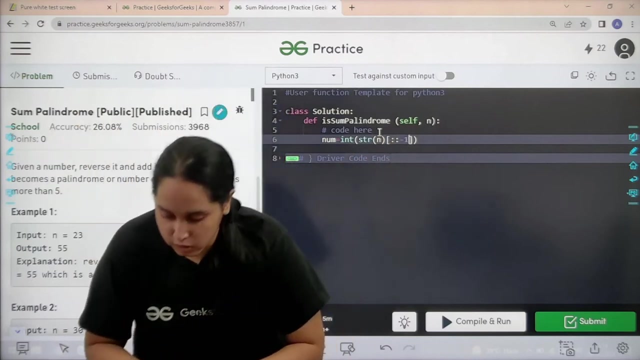 integer value of what? of the string n, and you are taking it the reverse right. You need the reverse of the given number as well, because you need to calculate the sum right, and the sum should be the original value plus the reversed value right. So that is what is you are doing over here. If now 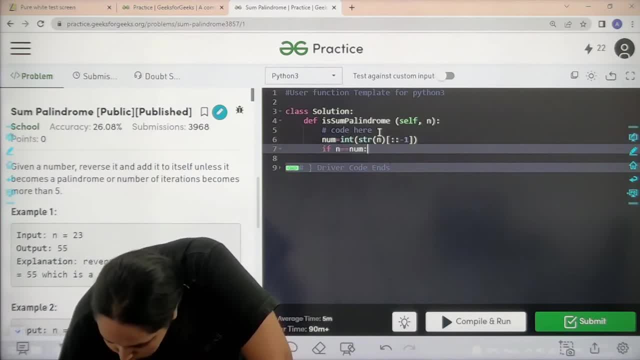 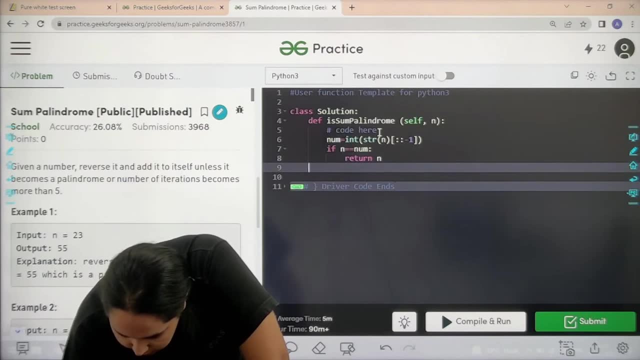 I am checking if both of them are equal or not. If both of them are equal, then you can just return it. Okay, after this, after this, you need to apply the for loop right because you need to check the palindrome right. I in range of what? in range of five right? You only have five iterations after. 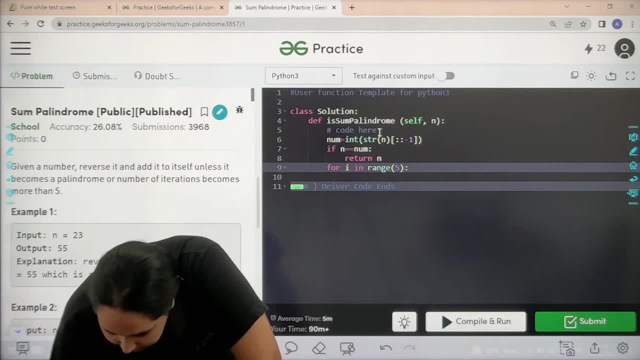 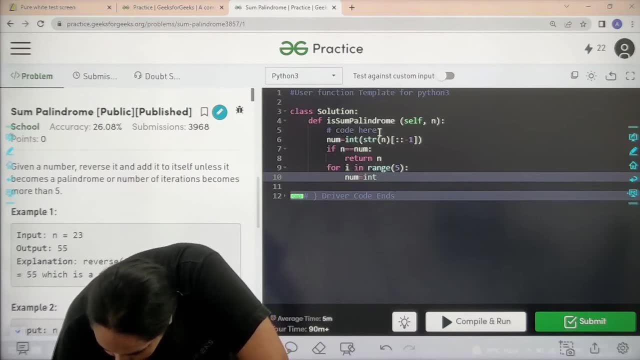 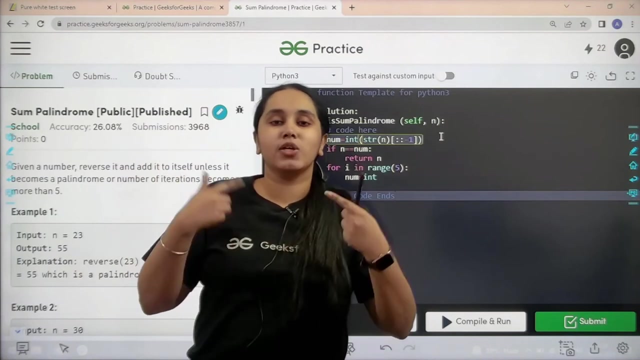 five iteration. you don't have any more iterations. right Then, num equal to int. again, you are calculating the same thing that you did above. right, You are calculating the reverse, because it is mentioned. You need to keep on reversing it again and again, and again and again. you need to keep on adding as. 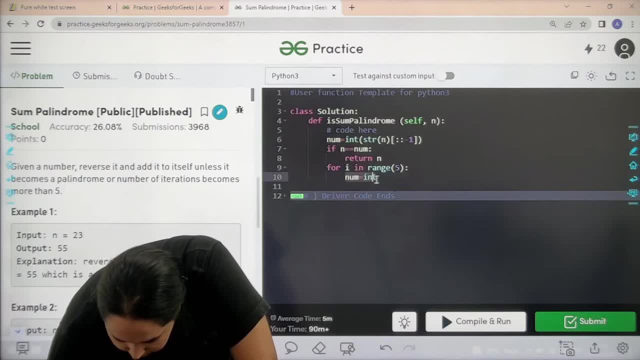 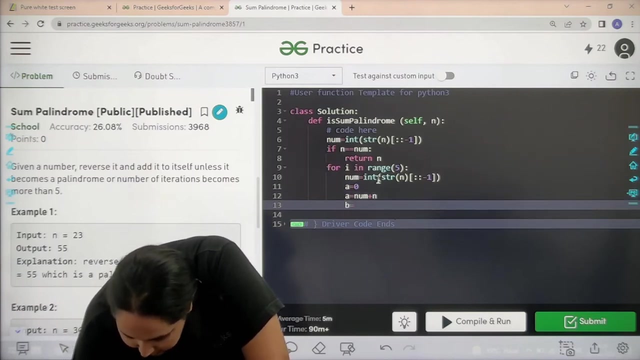 well, So let me just copy this and paste it here One minute, Okay. next, a is initially zero, then a is the sum right, A is the sum of the two values. Then next b. Okay, what is b? b is another. 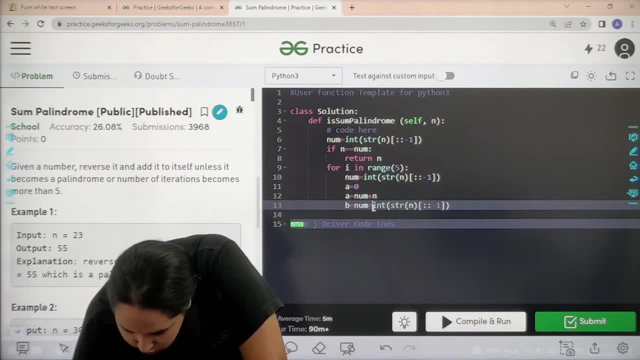 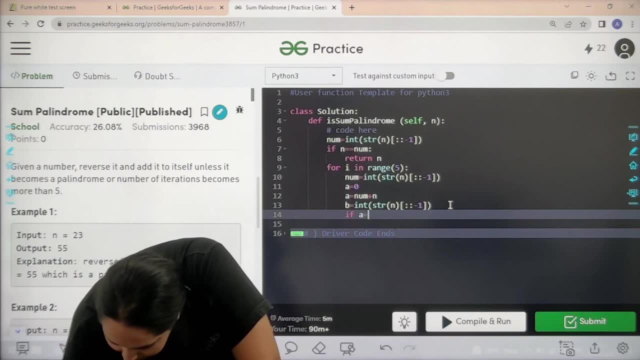 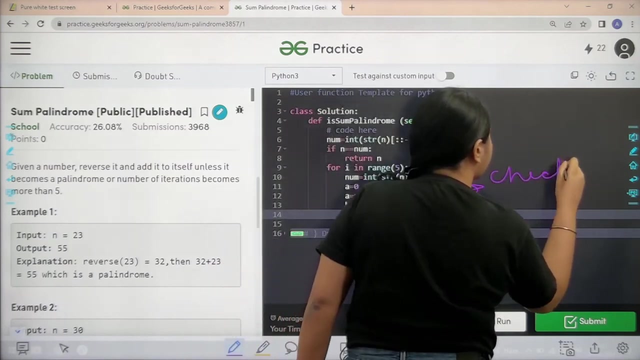 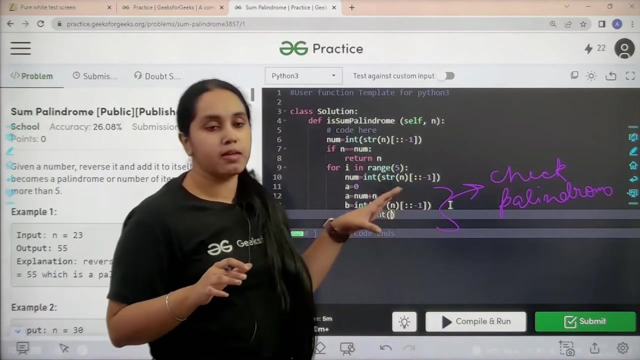 integer One minute with the reverse value, right? You need to keep on reversing it again and again. So reverse value. if a is equal, equal to integer of b. This b is declared to check palindrome. Okay, this b is created to check the palindrome. Okay, this b is created to check the palindrome and this: 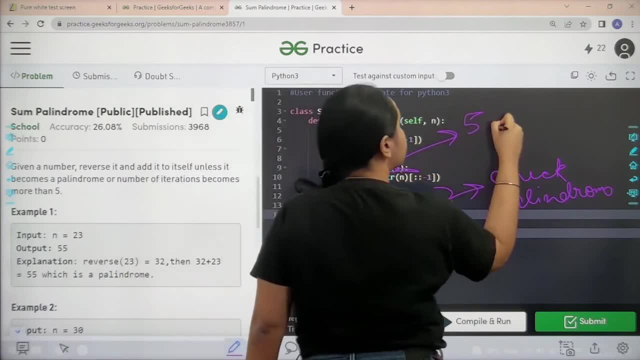 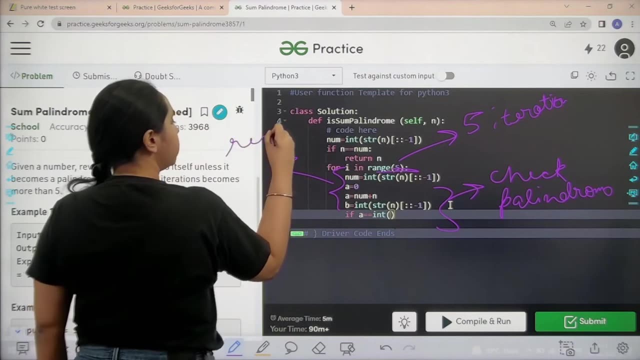 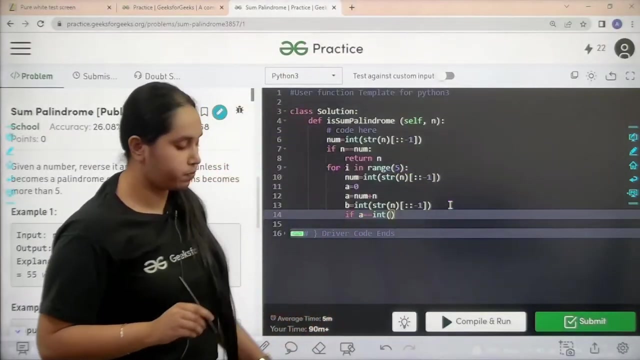 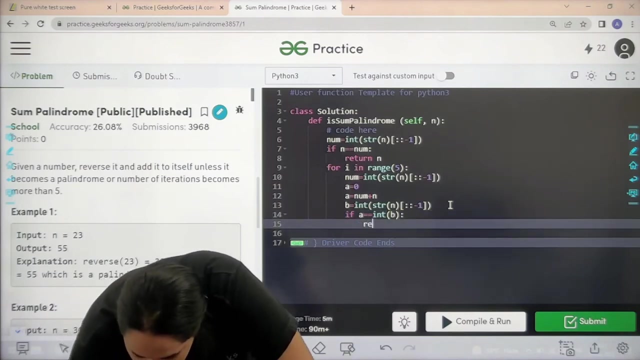 one. this is, you know, five iterations. You are specifying five iterations, Okay, and over here you are doing that: reversing And sum. Okay, you are doing reversing and sum. Okay, now let's continue. Integer of b, because you are comparing right. and then you need to return with a if they are correct, right, Else if they are not. 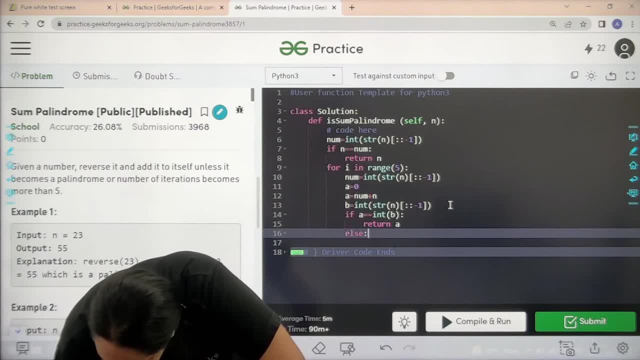 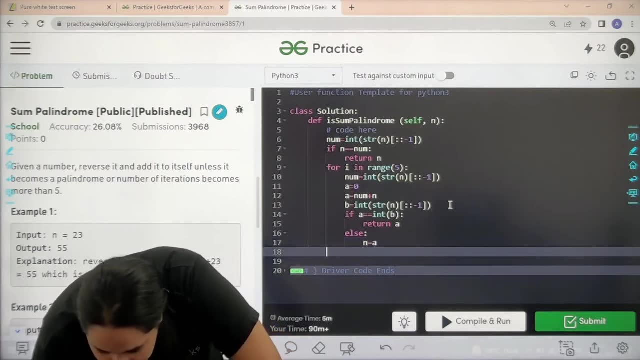 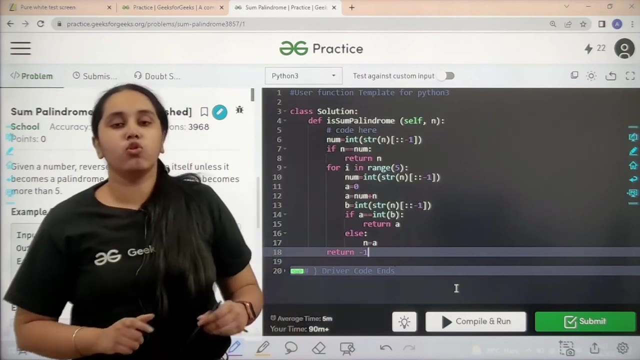 correct. you need to repeat the steps, right, Very good, After this. if this is not possible, right then you would just return with minus 1, because you know after five iterations are over you still didn't get the result. And now to check if it is correct or not, I would click on compile and run. Let's wait, It is getting.